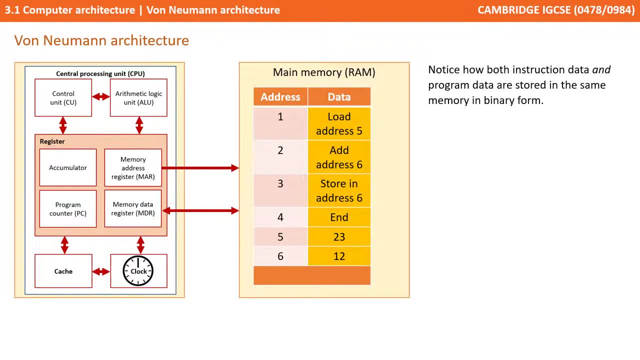 for processing. Let's have a closer look at the memory. You will notice that each instruction is stored in a location in the memory and each location has an address. Therefore, the processor can fetch an instruction stored in the memory- in memory address one, for example- and bring it back into the processor. Now 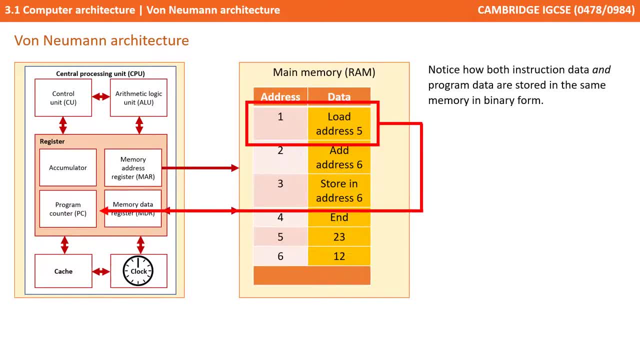 computers are complex machines capable of fetching and executing instructions billions of times a second, using a very methodical sequence of events inside the CPU. In order to do this, they make use of special purpose registers, which we introduced in the last video. Let's take a look at each one and see what it's. 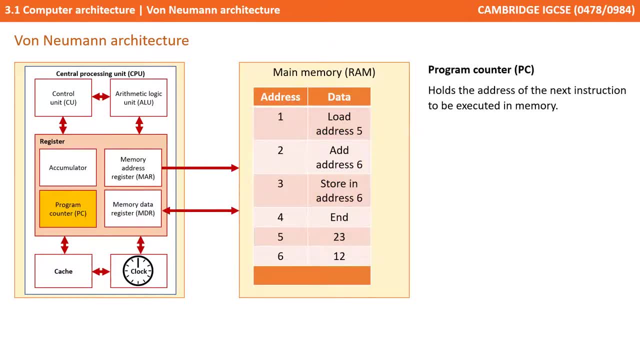 used for The program counter always holds the memory address of the next instruction to be executed. Once we fetch this address from the program counter, we increment its contents by one, so it points to the next instruction to be executed. The memory address register holds the address of where data is to be. 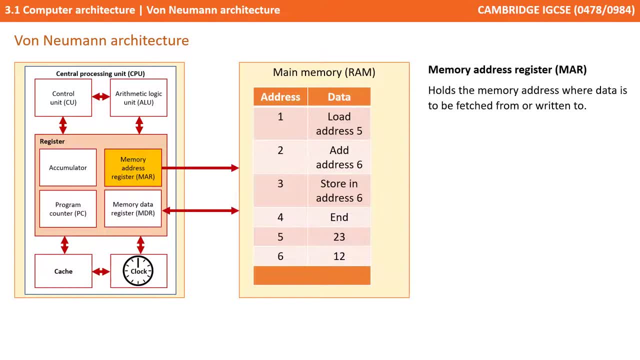 fetched from or stored into The memory data register holds any data which has been fetched from memory or is about to be written to memory. The accumulator holds the results of calculations which have been performed by the arithmetic logic unit. Let's look at a typical fetch execute cycle in a little more detail. So we start with the. 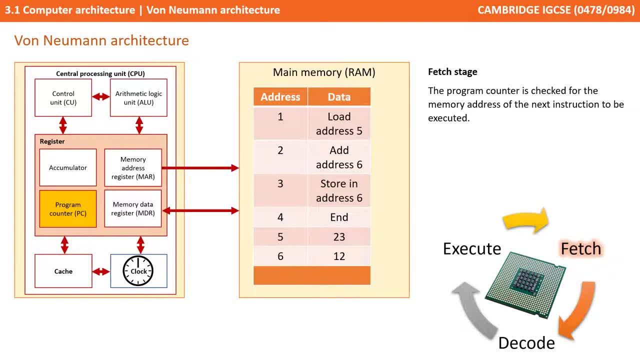 fetch stage, The program counter is checked As it holds the address of the next instruction to be executed. This address is used by the memory address register in order to fetch the instruction needed from main memory and bring it back into the memory data register. The address in the program counter is incremented to point to the 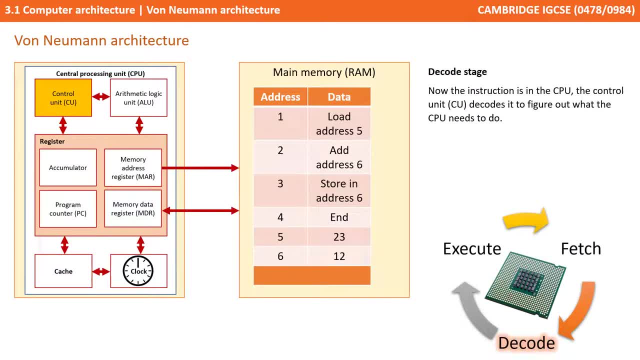 next instruction. Now the instruction is in the CPU. the control unit decodes the instruction to see what has to be done. Now we know what to do. we can execute the instruction. What we actually do depends on what the instruction actually is. We could be asked to head back to.